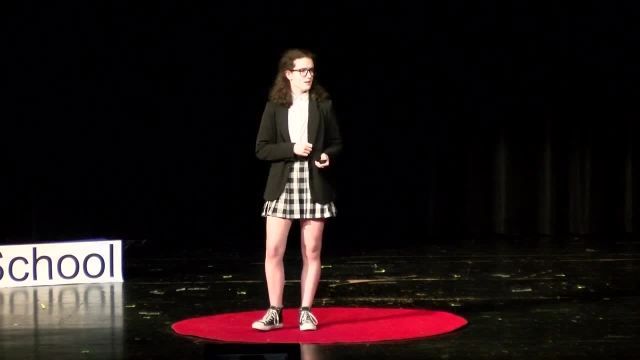 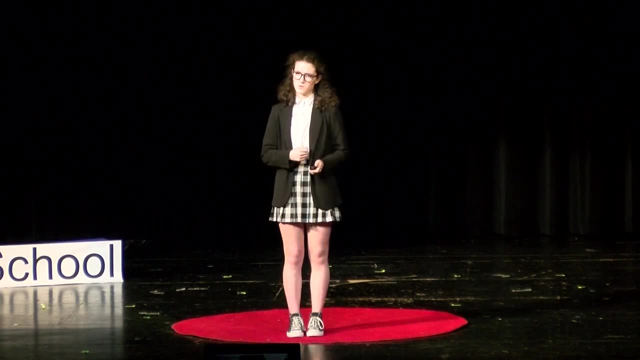 two or three weeks in February, And every year the summers are getting a little bit hotter and the winters are also getting a little bit hotter. We're seeing the effects of climate change right here in our own community, albeit sometimes it may be very subtle, like a few. 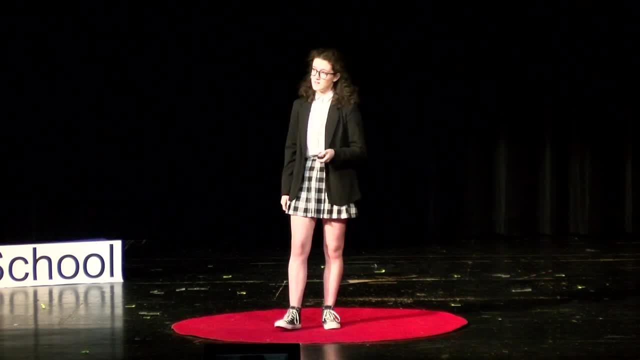 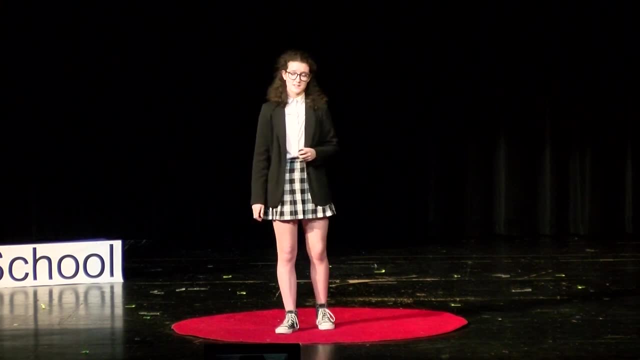 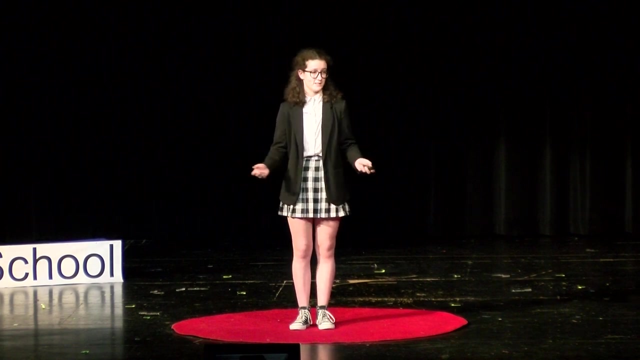 degrees on your summer pool party, But sometimes it's mid-February, the power's been out for days, temperatures are below freezing. you're bundled up in five blankets eating dry cereal and savoring the last percent of your phone battery. wondering: where did it all go wrong? Personal anecdotes. 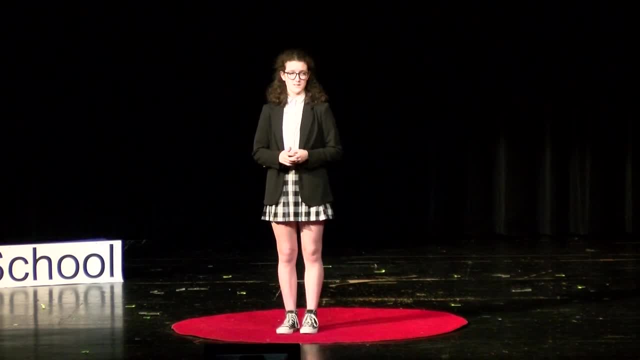 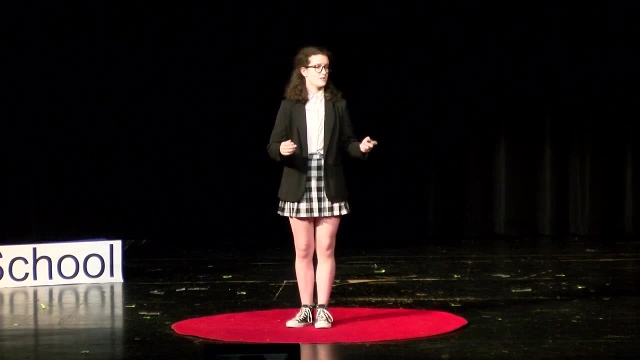 aside, climate change is a very important issue. Sea levels are rising, currents are changing, they're pushed out of their habitat and many are threatened with extinction. Storms that are supposed to happen every 500 years are becoming annual experiences. Climate change is a problem. 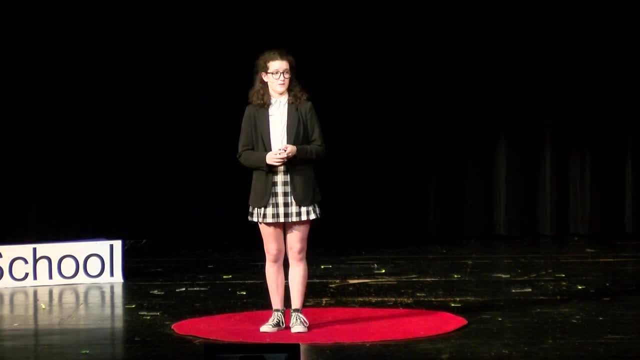 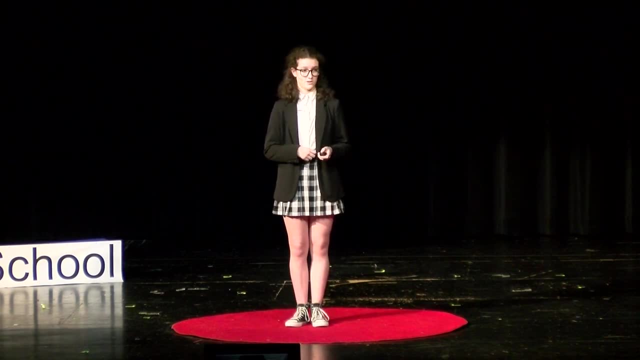 that will eventually affect every single person and thing on this planet if something isn't done about it. Today I'm here to discuss a brief history of climate change, as well as the human impact on it through emissions and education to hopefully involve some breaking-edge solutions. 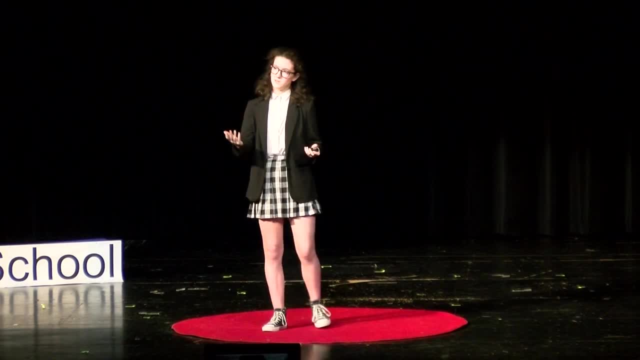 into our discussion Now. civilizations as far back as ancient times have been a part of the history of climate change, and they've been a part of the history of climate change. In ancient Greece. we're able to deduce that cutting down trees would. 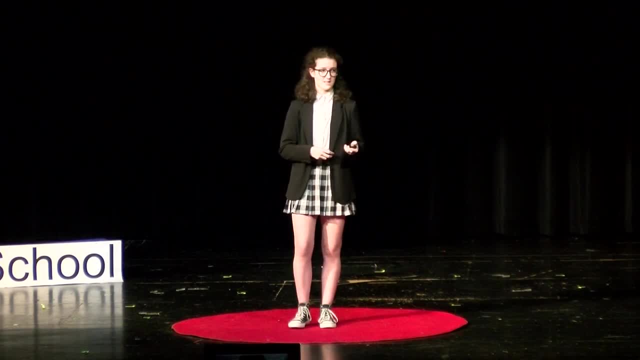 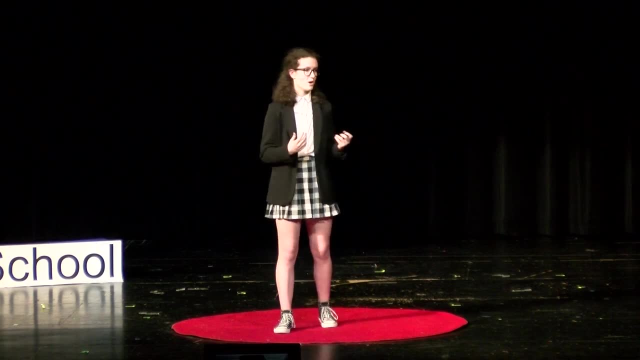 change rainfall and temperatures in an area, And NASA says that humans have been causing emissions for some time now, which is why it's so strange that this man was the first one to theorize that humans could possibly have an impact on our climate. He is Svante Artemis, a Swedish scientist. 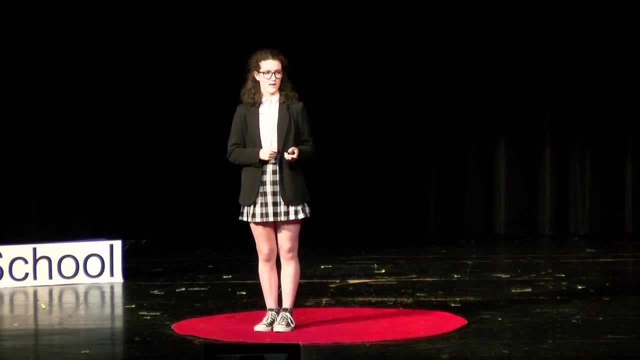 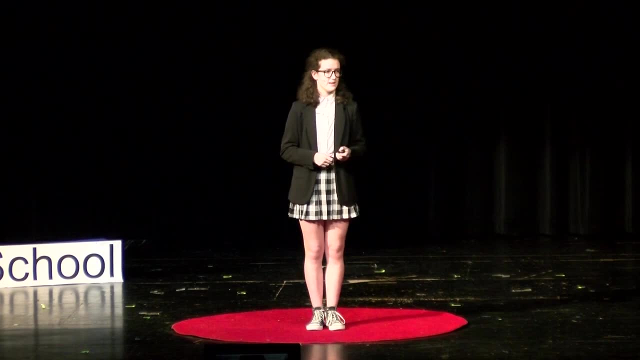 who first published this idea in an 1888 research paper and a follow-up paper in 1898, about how carbon could impact the environment. He theorized that when humans burn coal and natural gases, they release carbon dioxide And he said that if we could do that, we could do it. And he said that. 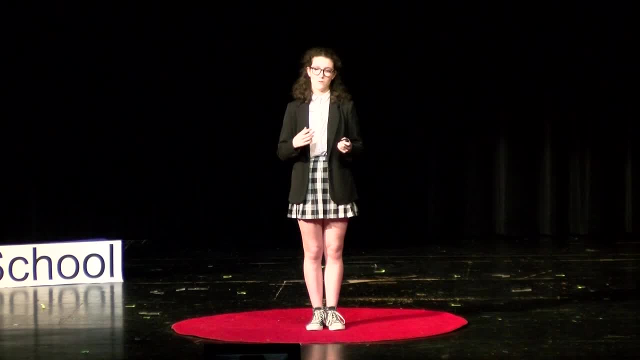 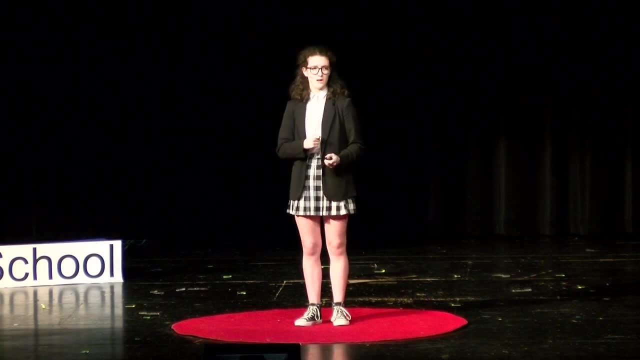 if we could do that, we could do it. And he said that if we could do it, we would reduce copper emissions and replace carbon, which can contribute to rising temperatures. Now this was a great opportunity for humans to catch this problem early and examine some solutions before irreparable. damage happened, Unfortunately for humans everywhere. people don't really enjoy to be blamed for things, so his findings were swept under the rug by the scientific community until much later, In the 1950s. extra funding from the Cold War allowed scientists to further look into problems. they 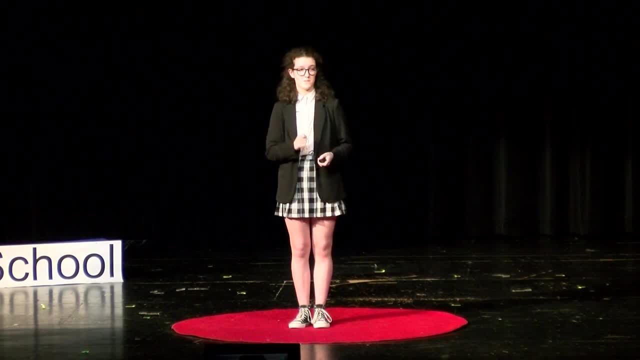 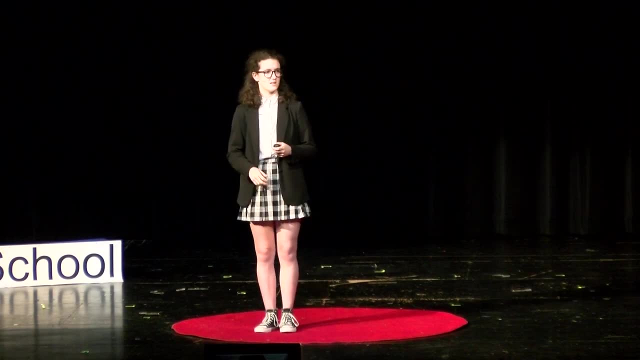 saw with warming in the North Atlantic regions, scientists finally had solid empirical evidence that could prove that human emissions could cause climate change. Now, even though scientists knew about this, it wasn't until environmentalist movements in the 1970s where the public became generally aware of the idea. 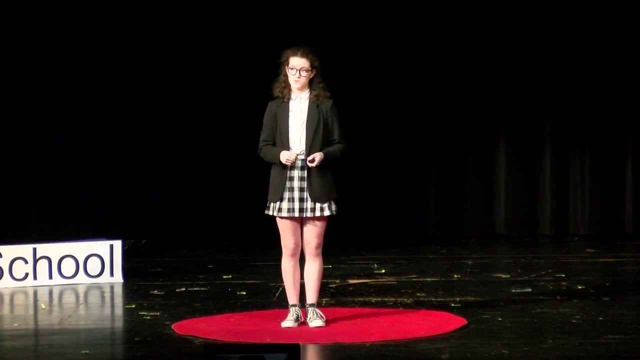 And international action wasn't taken until the late 90s and early 2000s, when the UN put together the Intergovernmental Panel on Climate Change. Still, there's a lot of education to be done. In fact, a study by the Royal Swedish Association of Scientists 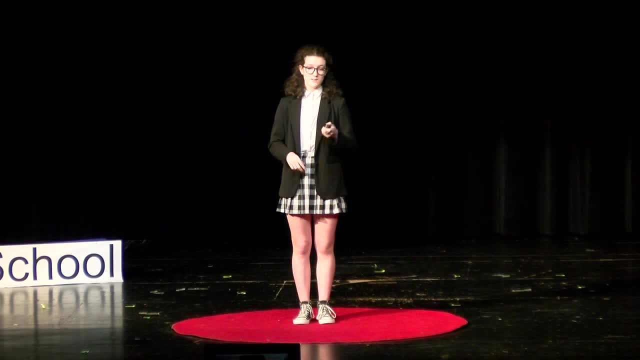 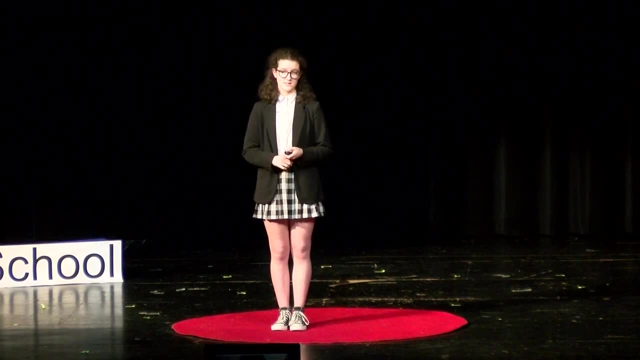 found that, of the high school students surveyed, only 79% believed that climate change was caused by humans and only 68% believed that it was an actual threat. This is because they weren't educated on the topic. In fact, after they took these opinions, 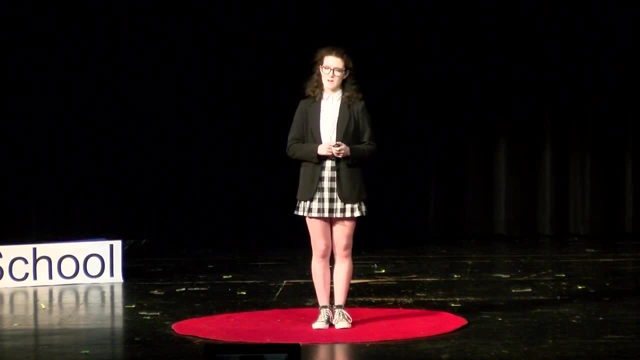 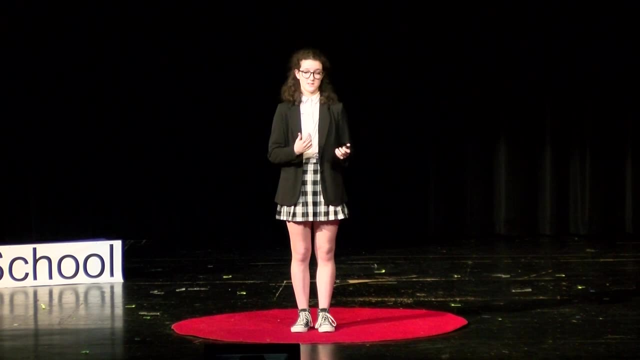 they administered a test about the science behind climate change and they found that those who held the belief that it was caused by humans and that it was a threat typically did much better on the test than did those who didn't believe those things. This shows a correlation between being educated. 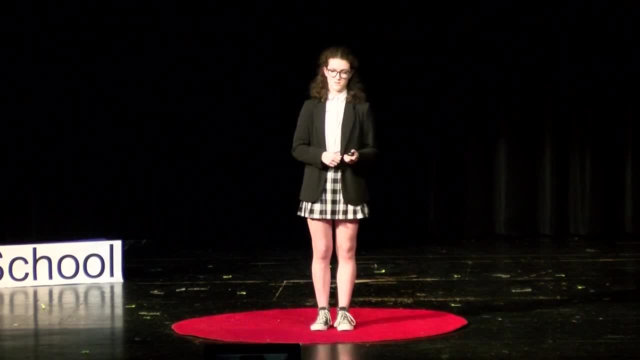 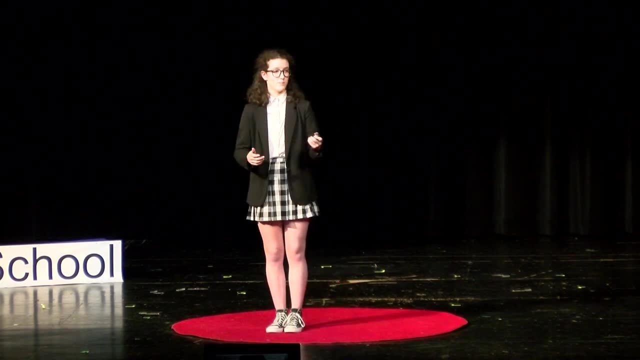 and being educated And being able to make accurate judgments about information. Now the solution to this problem is simple: Educate people, Educate kids from a young age. Make it a part of schools. Teach them about it from a very young age. 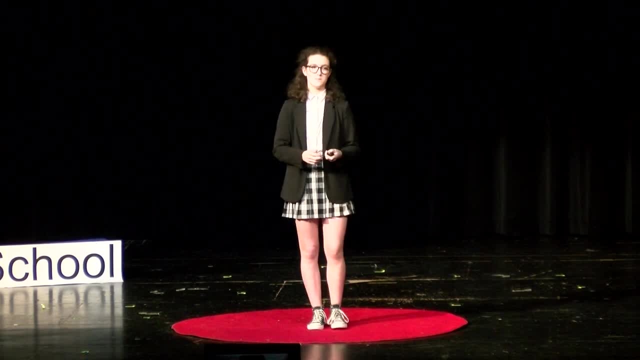 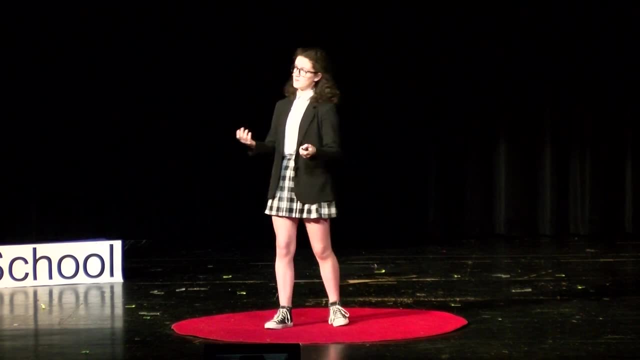 and once people become educated on the general idea, we can delve deeper, explore the specifics and hopefully come up with some nice solutions to this global problem. Even once people have a basic education, there are still some issues. People who agree that climate change is a problem. 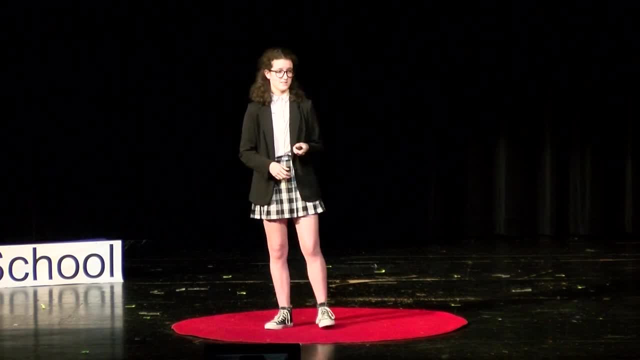 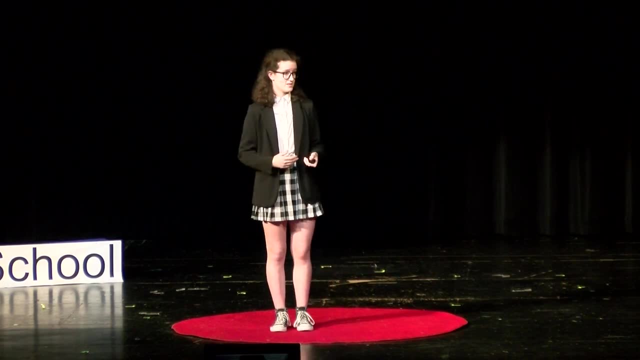 people who agree that climate change is a threat caused by humans still disagree on the extent to which humans cause it. I'm sure you've all seen the PSAs about single-use plastic, or don't waste the electricity, And while, yes, these are ways to reduce your personal carbon footprint, 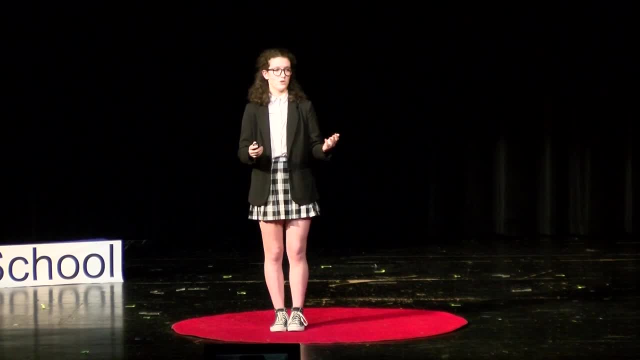 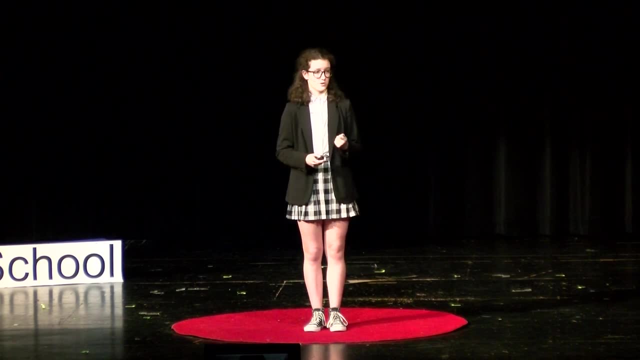 even if everyone was super vigilant about this, we still would only make a small dent in the huge problem that has human-caused climate change. The problem is people don't know where to look for the solutions, so they target the areas in which the effects are most clearly seen. That being underprivileged impoverished areas. For example, during Hurricane Katrina, lower-class impoverished neighborhoods were hit harder, while upper-class suburbs remained mostly intact. Similar things have happened in other hurricanes, like Hurricane Harvey and other 500-year storms that are becoming more and more common as our climate changes. 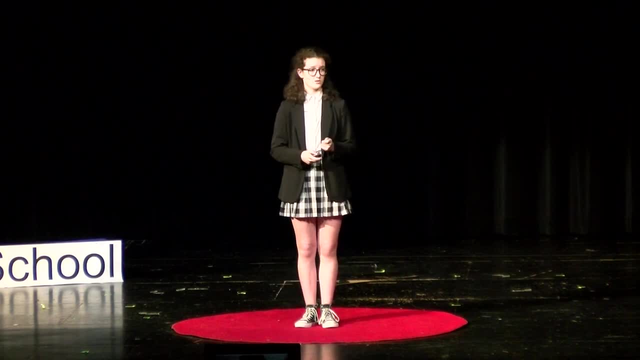 These individuals and communities are getting the brunt of climate-caused catastrophe and are thus being targeted when we talk about climate change prevention policies, when, in fact, the issues run much deeper than that. In a study by the Carbon Majors Database. 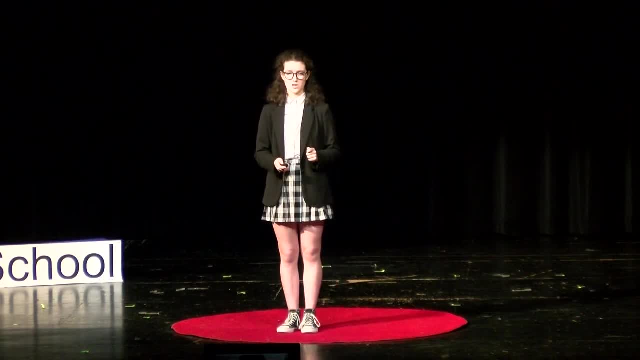 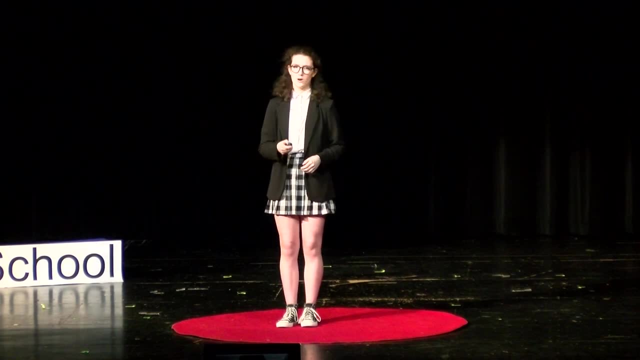 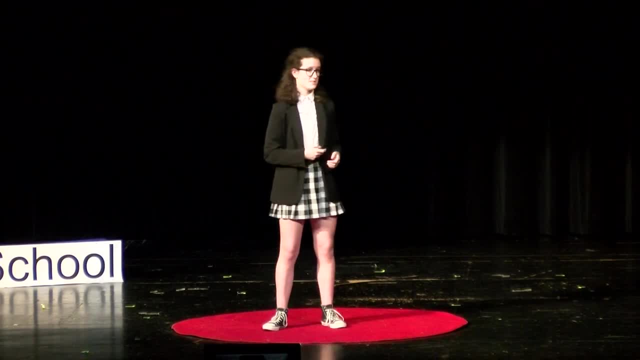 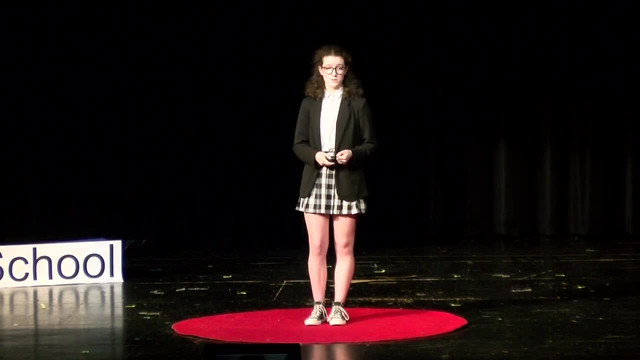 By 2050, companies could face $300 billion dollars of climate-caused carbon emissions, And they're realizing this. They've begin to shift their polices to hopefully make this a better. but what if this doesn't come soon enough? Well, scientists have come up with a way. 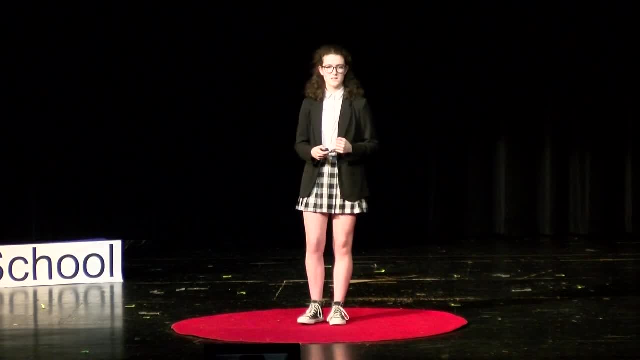 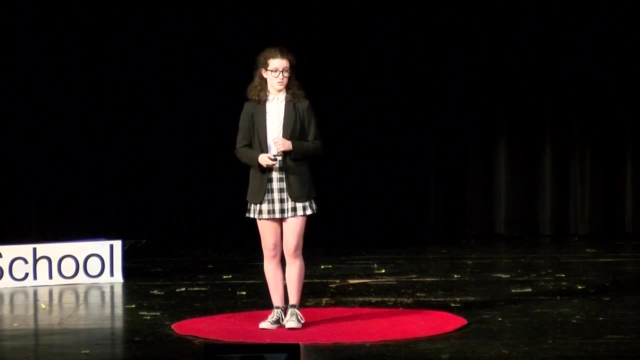 to hopefully take carbon out of the atmosphere. Carbon capture is a really effective way to reduce carbon emissions at some of our choke points like power points and factories. There's two ways to do this: precombustion and postcombustion. 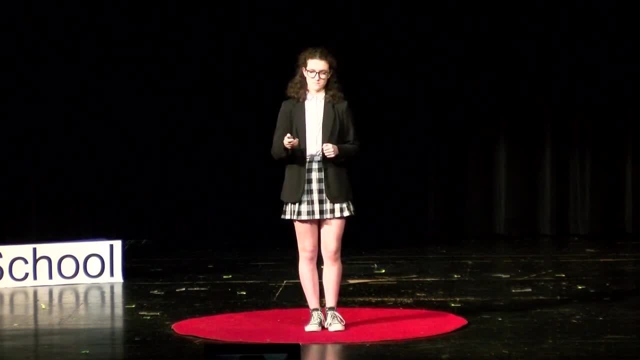 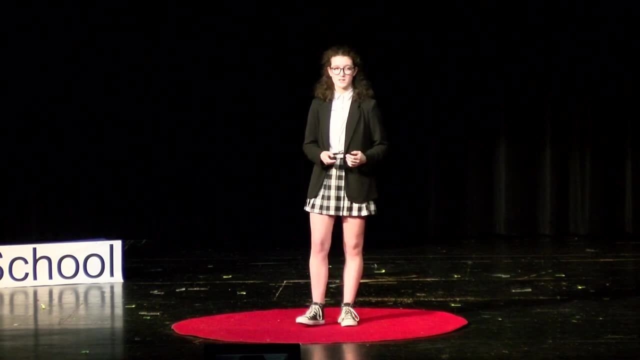 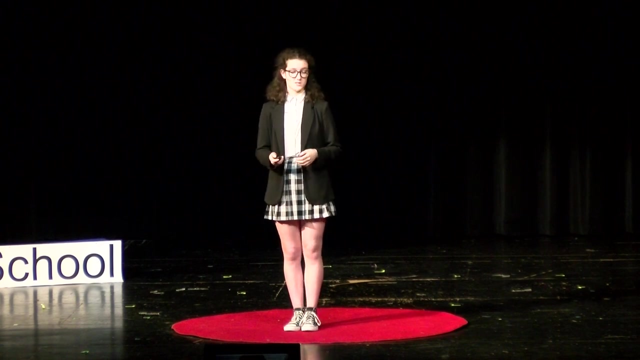 You can take the carbon out before or after the reaction happens. ambient filters are put over smokestacks and emission areas in factories to filter out carbon dioxide from reaching it to our air, And in pre-combustion, the gas, before it's burned, is put through a reaction to remove the carbon dioxide, so it never enters the reaction in the first place. 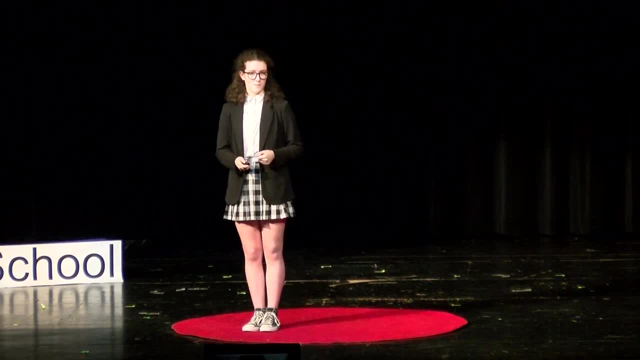 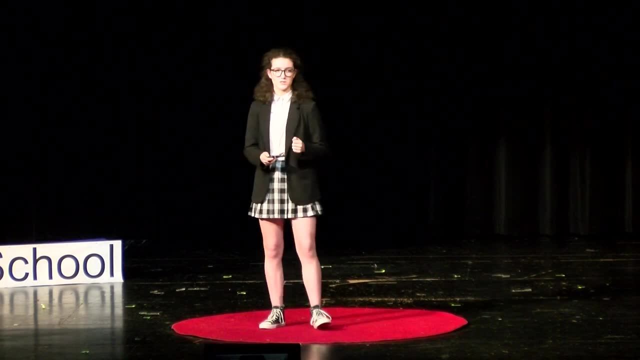 Now, this is all useful information, but what are we going to do if we can't capture that carbon we removed from the reaction? This is an important part if we want to curve these emissions. Carbon becomes increasingly difficult to capture the farther it gets away from its source point. And the methods to do this are very expensive and would need to be widely implemented in a short amount of time to be effective. So what do we do? Well, a company called Carbfix is hopefully coming up with a solution for this, called carbon mineralization. It's where they dissolve carbon in water and then inject it into basaltic rocks or other reactive rocks to permanently solidify and mineralize it and reduce it from reentering the atmosphere. They start their trials in 2022 to hopefully offer companies a more effective and cost-efficient way to reduce carbon emissions. 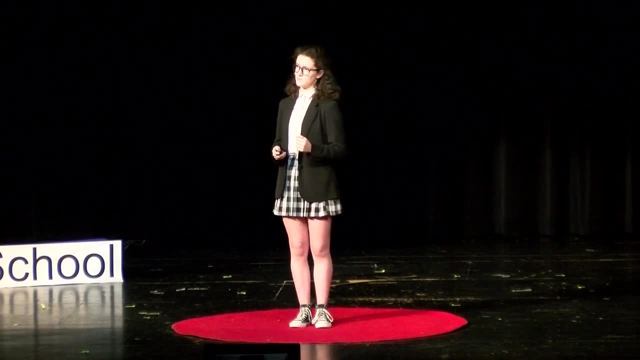 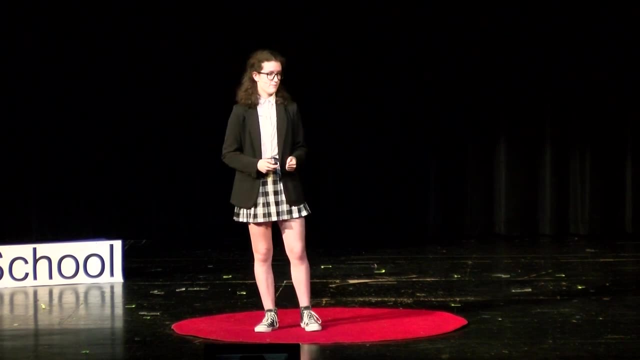 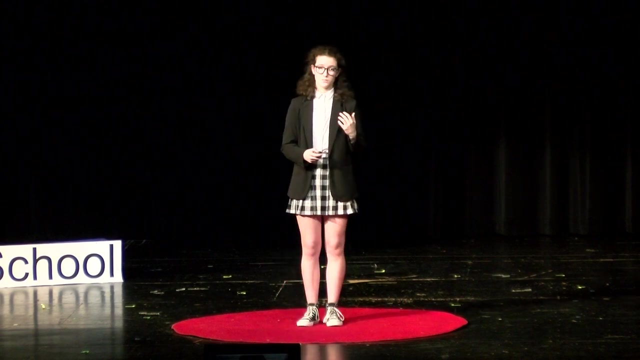 Even with all this science, the most effective way to stop these false informations is to be aware. Raise awareness, put out accurate information, Because climate change doesn't get nearly enough attention for how big of a problem it is. Our biggest tool is to raise awareness and to advocate to do the right thing.